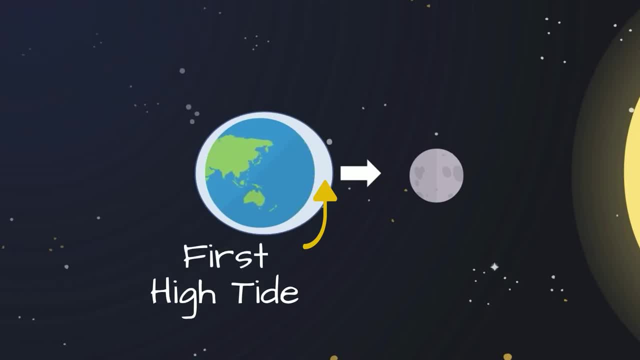 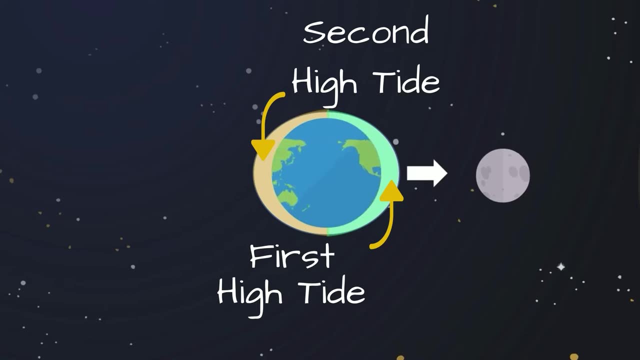 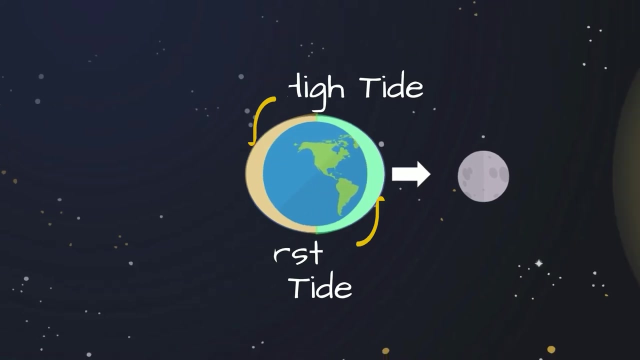 as the first high tide. the second high tide, or the bulge on the far side of the earth, is caused by inertia. the second high tide is a result of a counterbalance to the pull of gravity from the moon. you can also think of the earth as being squeezed and embolging on both sides. as the earth. 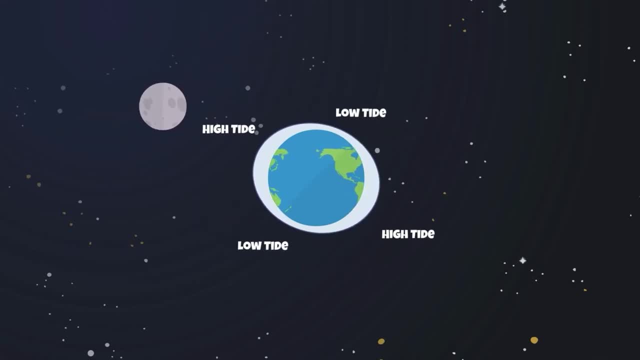 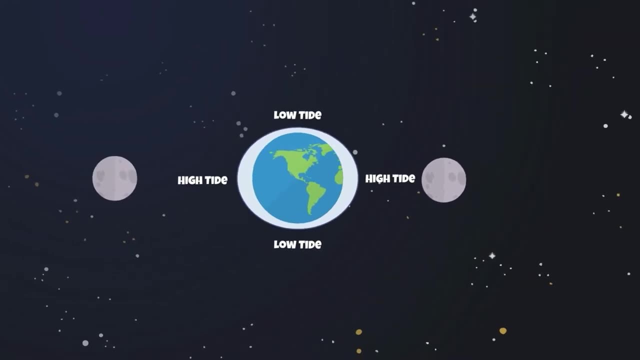 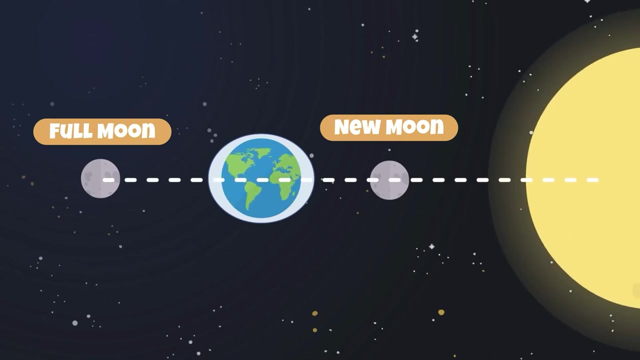 rotates. there are patterns in high and low tides throughout the day. these patterns can also be seen during a lunar cycle. in both the new and a full moon, there's an alignment of the sun and the moon to the earth, creating a combined gravitational pull. this combined pull causes 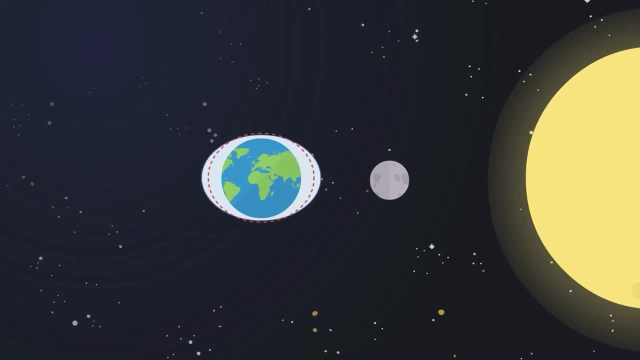 the water in the earth to bulge more than usual, causing higher tides, or what are known as spring tides. it takes the moon seven days after a spring tide to orbit around the earth and form a right angle in its position to the sun. this is when neap tides are formed. in a neap tide, the gravitational pull of 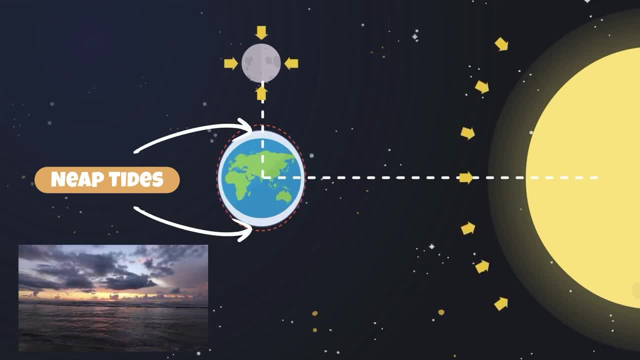 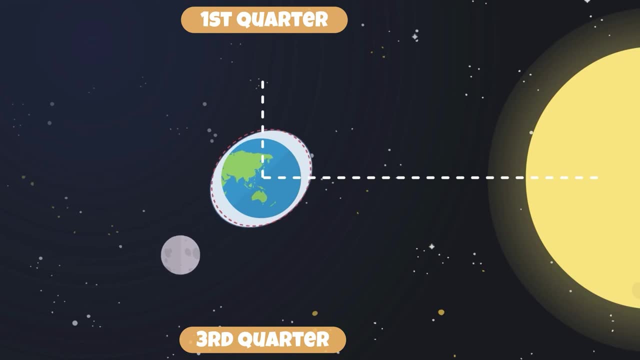 the sun counteracts that of the moon, forming moderate tides. neap tides occur at the first and third quarter phase of the moon. this is where the moon's orbit around the earth is perpendicular to the sun you. it takes the moon approximately one month to complete one revolution around the earth. 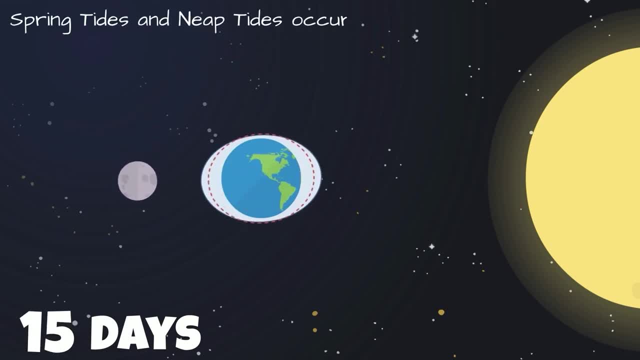 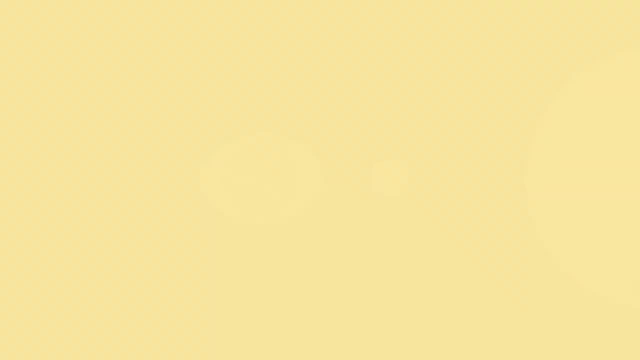 this means that both spring tides and neap tides occur twice in a lunar month. let's review we just learned: high and low tides are caused by the gravitational pull of the moon on the earth. the first high tide is caused by the earth rotating into a bulge of water. 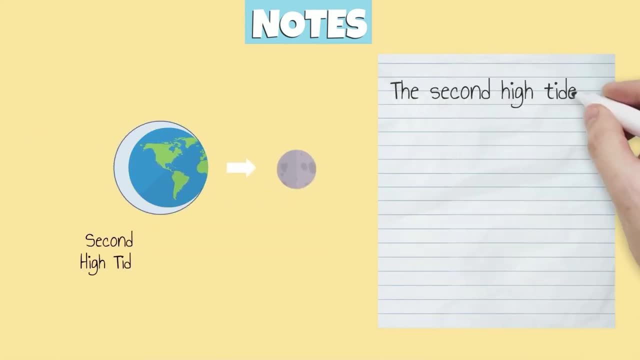 caused by the gravity of the moon, and the first high tide is caused by the earth rotating into a bulge of water, where it has free movement and responds to the hardships and storms caused by gravity of the moon. the second high tide occurs on the opposite side of the earth and is caused bye inertia or by the.